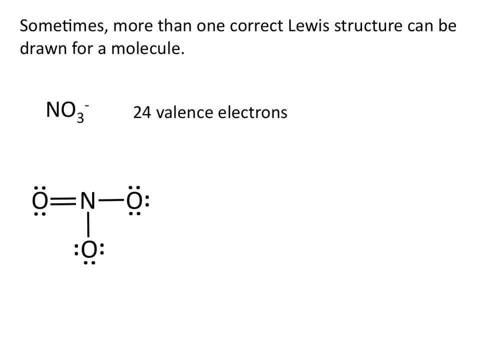 But did I have to move the electrons from the oxygen on the left to create a double bond? And the answer is no. I could have moved. I could have created a double bond between nitrogen and any of the oxygen atoms, And these equivalent structures are called resonance structures. 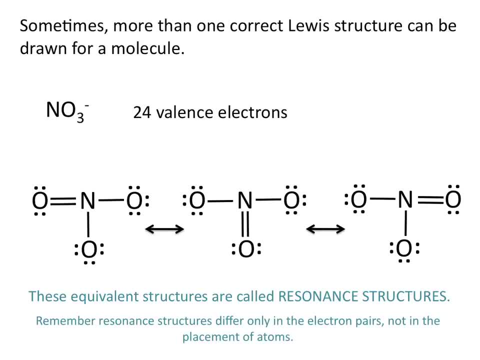 Something that's important to remember is that resonance structures differ only in the electrons that are on the left, And these resonance structures differ only in the electrons that are on the right electron pairs, and not in the placement of atoms. If you change the placement of atoms, 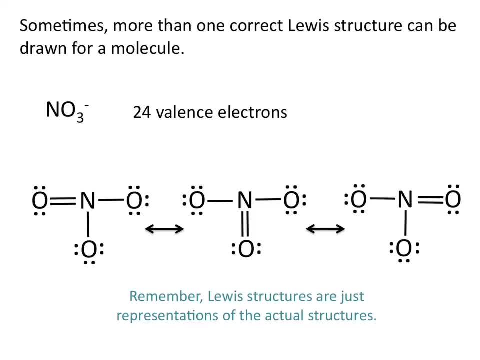 then you're changing the actual molecule. The other thing to remember is that Lewis structures are just representations of the actual structures, And so the actual structure is a hybrid of these resonance structures. So if I had a collection of NO3 minus molecules, I wouldn't see the double bond between nitrogen and oxygen. 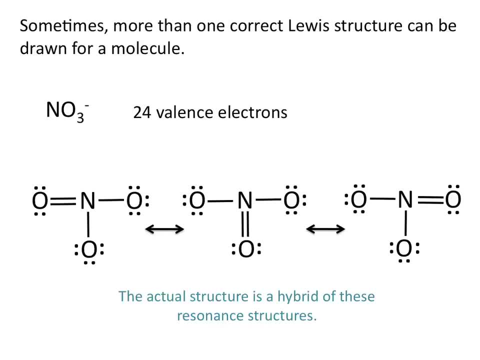 in varying positions. In fact, I would see all equivalent bonds between the nitrogen and oxygen atoms, And this is because, instead of that double bond existing between one nitrogen and one oxygen atom, it's actually shared between all three oxygen atoms, And so it's sometimes helpful to compare resonance structures. 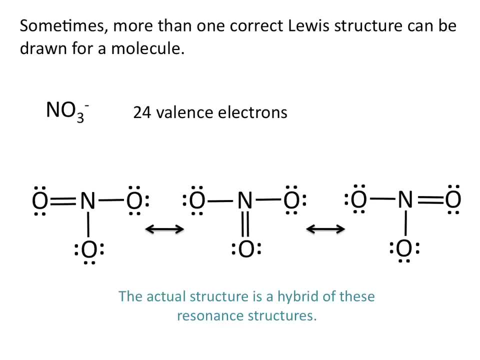 to mixing different colors of paint. For example, if I were to mix red paint and blue paint, I wouldn't have paint that oscillates between red and blue, being red sometimes and blue sometimes. I would have paint that was purple, that was. 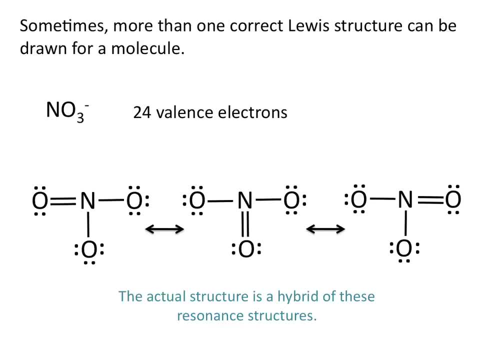 a mixture of the two colors, And it's the same way with resonance structures. I don't see this double bond switching positions in different molecules. The structure is actually a hybrid of these three structures And we just draw them all out separately to represent this. 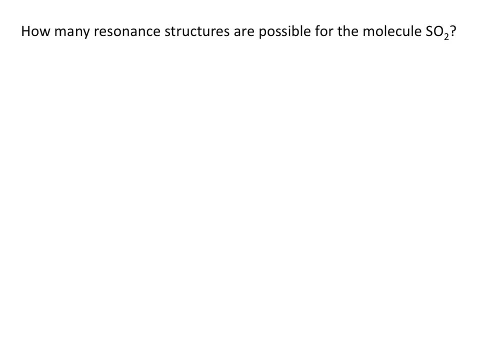 How many resonance structures are possible for the molecule SO2?? SO2 has 18 values And it has 18 valence electrons. When we draw the structure for SO2, we start by placing the central atom in the middle and draw it bonded to each of the oxygen atoms. 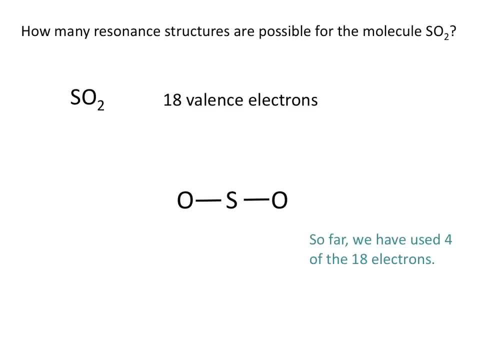 Remember that there are two electrons in each bond. So as of now, I've used four electrons. Then I start by filling in the octets of the remaining atoms, saving the central atom for last. So this structure includes all 18 valence electrons.